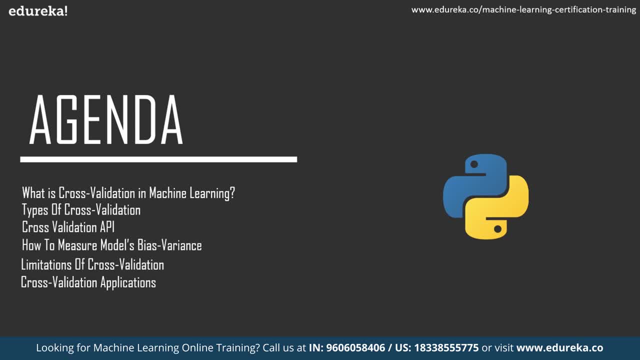 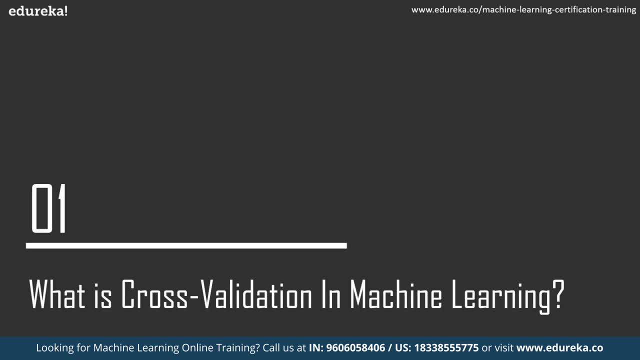 from edureka also. do check out the edureka's machine learning certification program. The link is given in the description box below. now, without any further ado, let's understand cross-validation in machine learning. So what exactly is cross-validation for any model in machine learning? 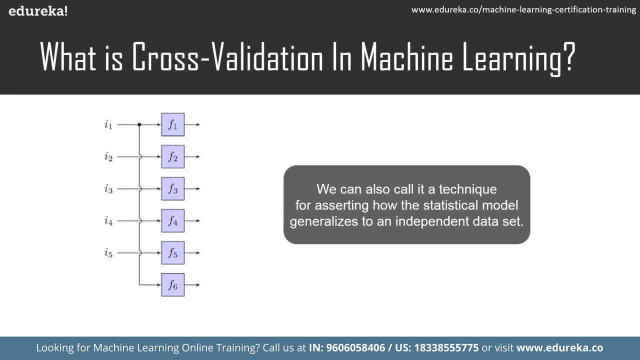 It is considered as a best practice if the model is tested with an independent data set. normally, any prediction model work on unknown data set, which is also known as the training set, but in real life scenario, the model will be tested for its efficiency and accuracy with an altogether different and unique data set. 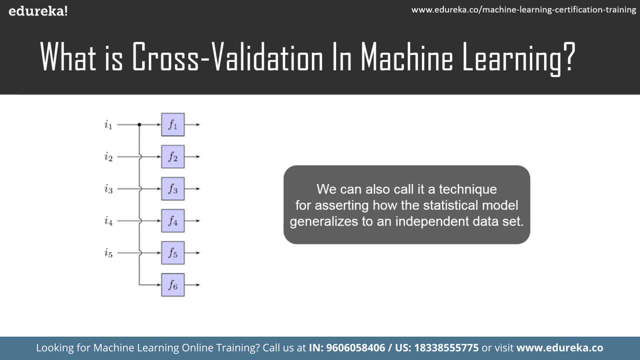 under those circumstances, You would want your model to be efficient enough, or at least to be at par with the same efficiency that it shows for the training set. So basically, this testing is known as cross-validation in machine learning, so that it is fit to work. 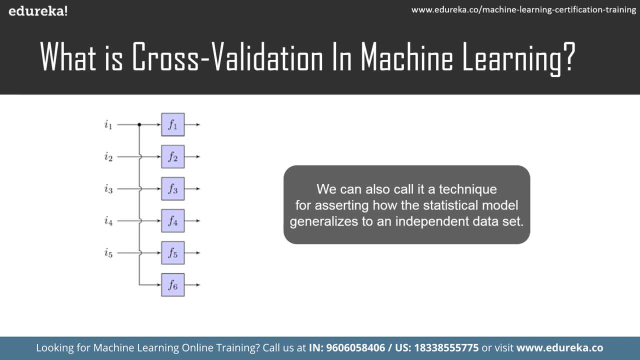 with any model in the future. We can also call it as a technique for asserting how the statistical model generalizes to an independent data set. So now that we actually know what cross-validation stands for, let us understand its importance in machine learning as well. 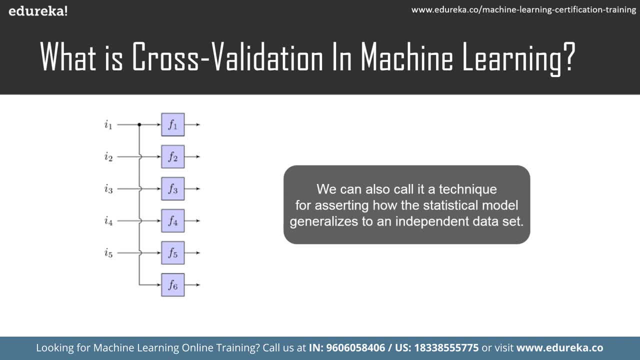 So let's try to understand cross-validation in simple terms. The basic purpose of cross-validation is to assess how the model will perform within unknown data set. So imagine you are trying to score a goal in an empty goal. It looks pretty easy and you could even score from a considerable distance too. 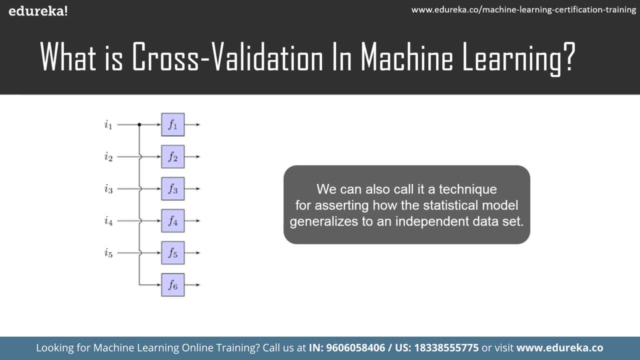 but the real test actually starts when there is a goalkeeper and a bunch of Defenders. So that's why you need to be trained in a real match, facing all the heat and still score the goal in the same case, with the statistical model. It is trained in such a way. 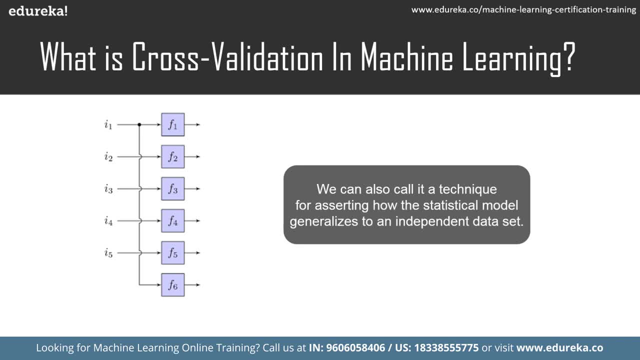 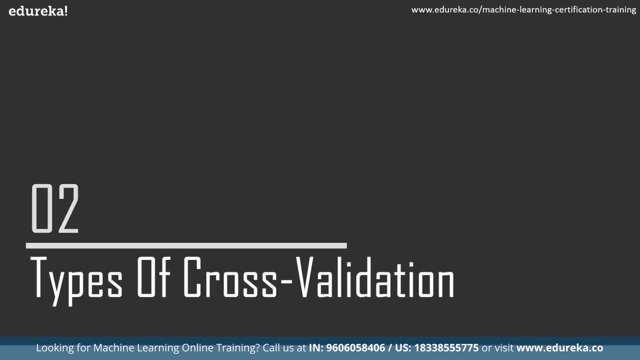 that it excels in its efficiency with other unknown data sets using cross-validation. So that is all about cross-validation. guys, Let's take a look at what are the different types of cross-validation. So there are basically two types of cross-validation techniques in machine learning. 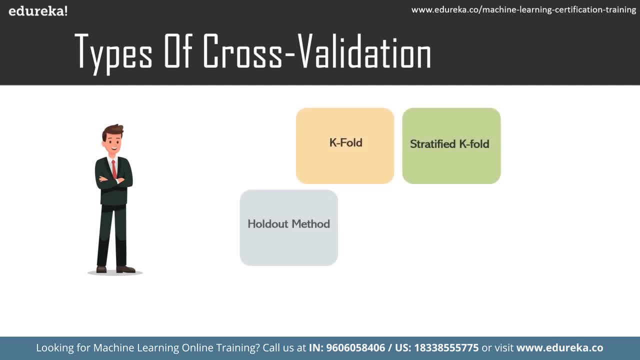 First one is exhaustive cross-validation. So this method basically involves testing the model in all possible ways. It is done by dividing the original data set into training and validation sets. For example, we have leave P out cross-validation and leave one out cross-validation. 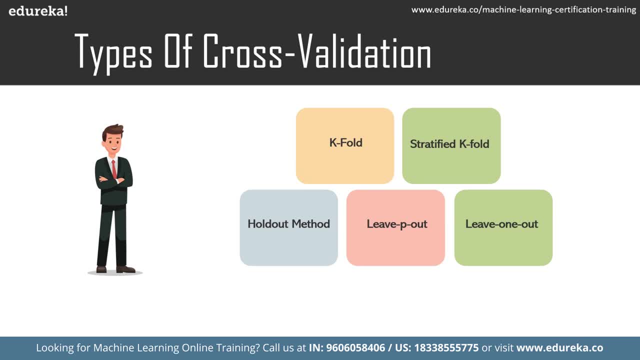 The other one is non-exhaustive cross-validation, and in this method the original data set is not separated into all the possible permutations and combinations. For example, we have k-fold cross-validation, holdout method, Etc. So let's talk about all these different techniques one by one. 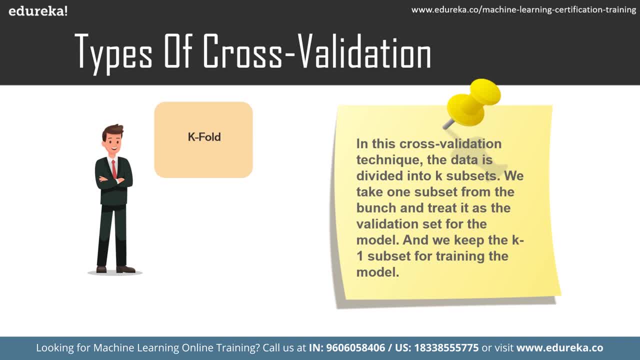 So first of all, let's talk about k-fold cross-validation. in machine learning, There is never enough data to train the model, and even then, if we remove some part of the data, it poses a threat of overfitting the machine learning model or it may not recognize a dominant pattern. 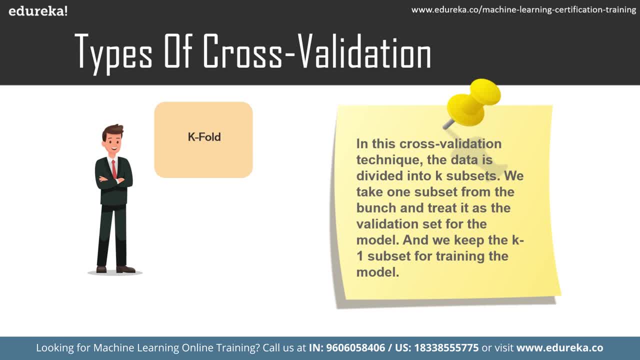 If not enough data is provided for the training phase. So by reducing the data, we also face the risk of reduced accuracy due to the error induced by bias, and to overcome this problem We need a method that would provide ample data for training and also keep some amount of data for testing as well. 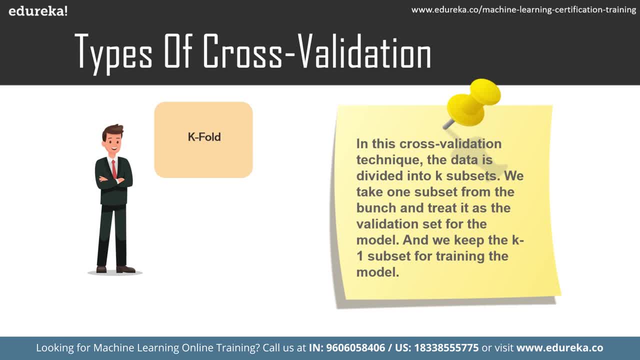 So k-fold cross-validation does exactly that. So let's talk about how exactly it works. So in this cross-validation technique, that is, k-fold cross-validation, the data is divided into case upsets and we take one subset from the data and treat it as the validation set for the model. 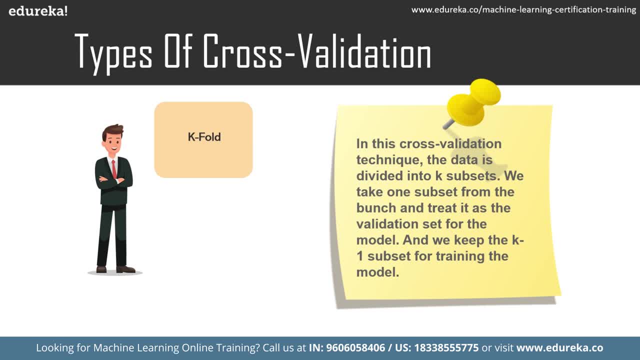 and after this we keep the key minus one subset for training the model. So the error estimation is averaged for all the K trials to get the effective readiness of the model. and each case upset will be in the validation set at least once, so it is also included. 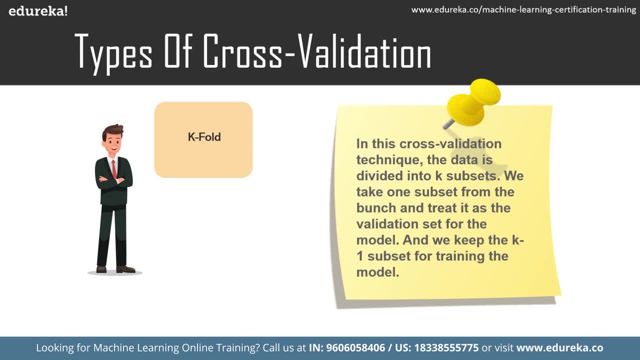 in the k-1 training set at least once as well. This significantly reduces the error induced by bias, and it also reduces the variance, as each of the case upsets is actually used in the validation as well. So this is how we can perform k-fold cross-validation. 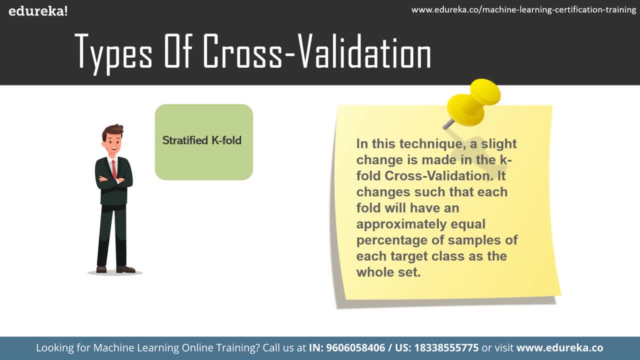 Let's talk about the next one that we have, which is stratified k-fold cross-validation. So in this technique a slight change is made to the k-fold cross-validation. it changes such that each fold will have an approximately equal percentage of samples of each target class as the whole set. 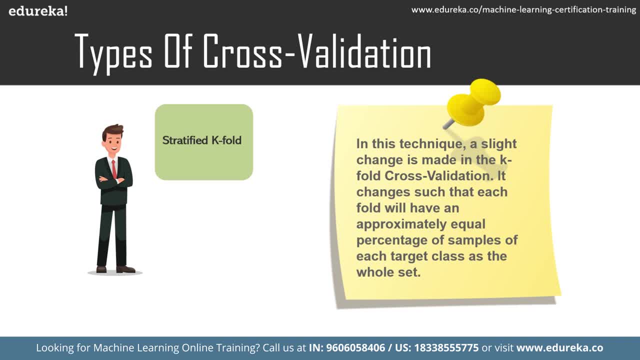 or in case of prediction problems. The mean response of value is approximately equal in all of the folds and in some cases there is a large imbalance in the responsive variables. Let's try to understand this with an example. So let's say we have a housing price example. 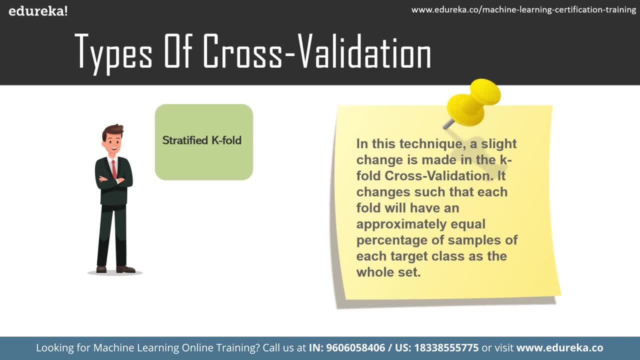 So the prices of some houses can be much more than the other houses, or in any classification problem, The samples may have more negative examples than the positive examples. So to tackle this discrepancy we follow the stratified k-fold cross-validation technique in the machine learning. 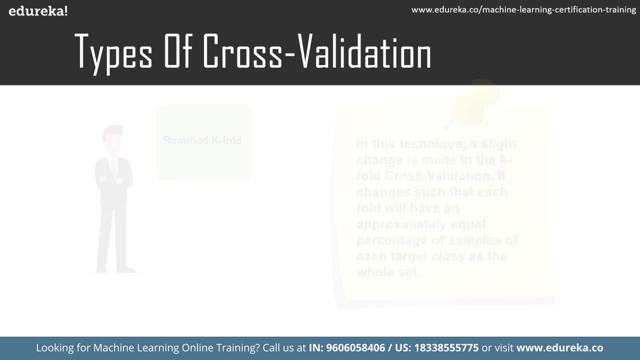 So that is all about stratified k-fold cross-validation. Let's talk about the next technique. It's holdout method. So this is the simplified cross-validation method, and in this method we randomly assign data points to two data sets. the size is not relevant in this case. 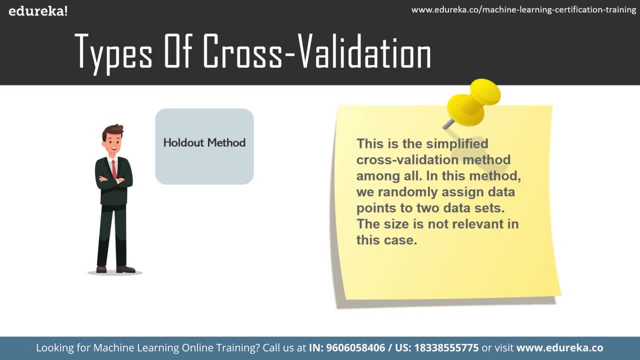 and the basic idea behind this is to remove a part from your training set and use it to get predictions from the model that is trained on the rest of the data. This method suffers from high variance, since it takes only a single run to execute all of this. 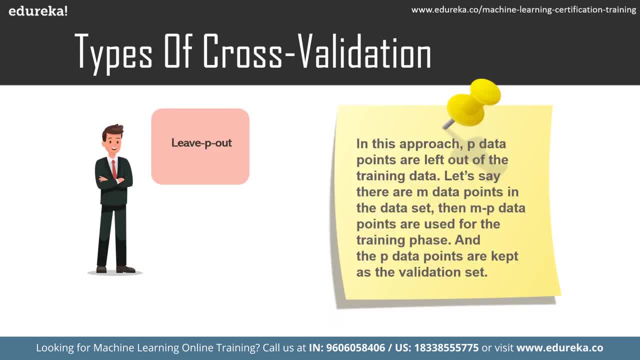 and it may also give misleading results as well. So let's talk about leave P out, cross-validation now. So in this approach, P data points are left out of the training data. So let's say there are M data points in the data set, then M minus P data points are used for the training phase. 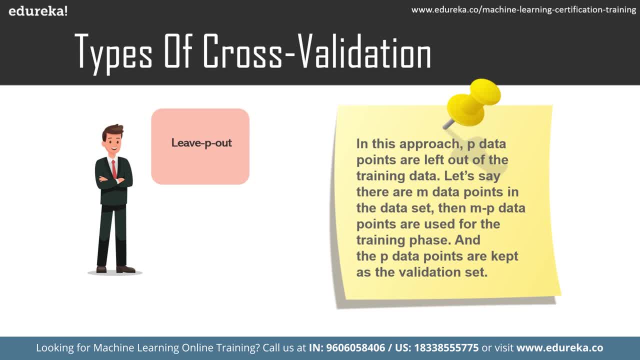 and the P data points are kept as the validation set. So this technique is rather exhaustive because the above process that I've just told you about is repeated for all the possible combinations in the original data set. and to check the overall effectiveness of the model, the error is averaged for all the trials. 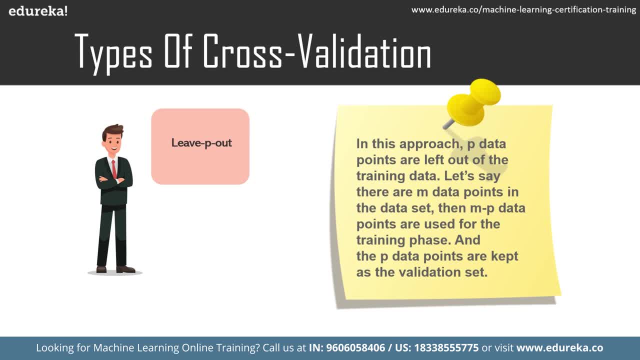 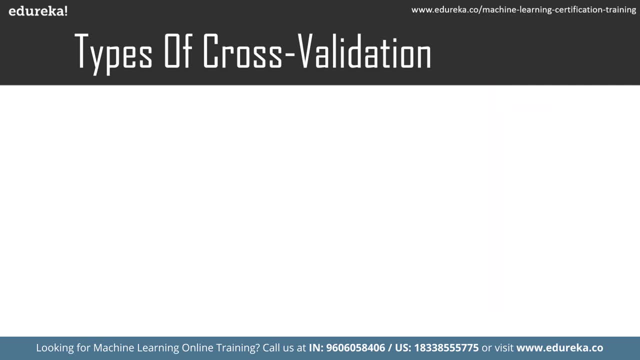 and it becomes computationally infeasible, since the model needs to train and validate for all the possible combinations and for a considerably large P as well. and then we have the leave one out cross-validation. This method of cross-validation is similar to leave P out. 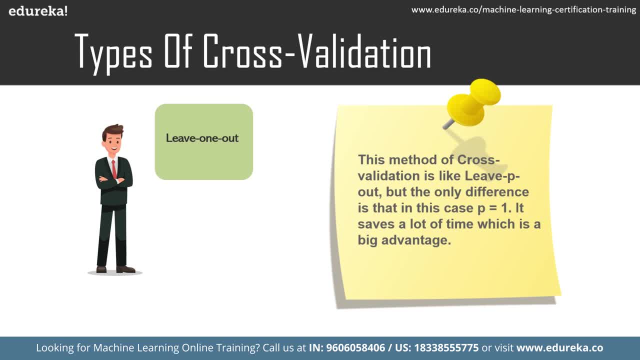 But the only difference is that in this case, P is going to be is equal to 1, and it actually saves a lot of time, which is a big advantage, Although when the sample data is too large, it can still take a lot of time. 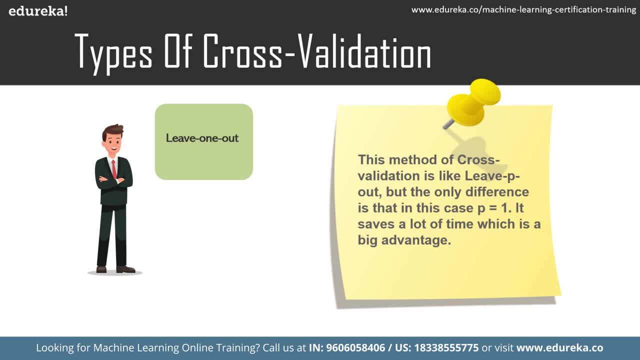 but it will still be quicker than the leave one out cross-validation method. And now that we have discussed the different types of cross-validation techniques, Let us take a look at the cross-validation API as well, So we do not have to implement cross-validation manually. 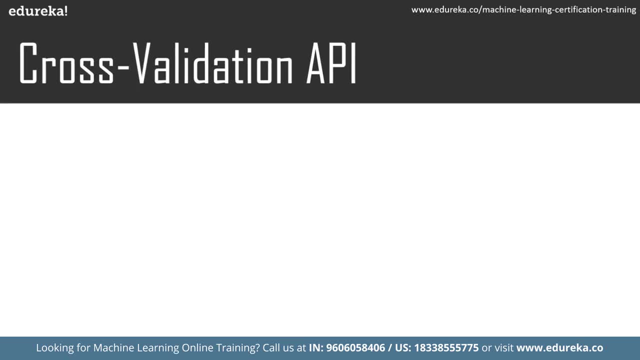 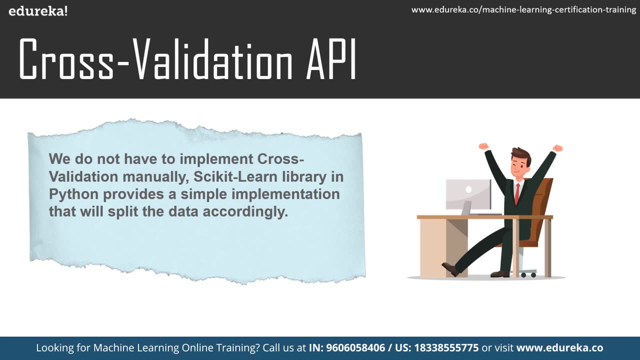 cyclic learn library in python provides a simple implementation that will split the data accordingly, and there are cross-validation iterators that are used depending upon the various cross-validation strategies. for example, for k-fold cross-validation We have a k-fold scikit-learn class. Similarly, we have leave one out class for scikit-learn. 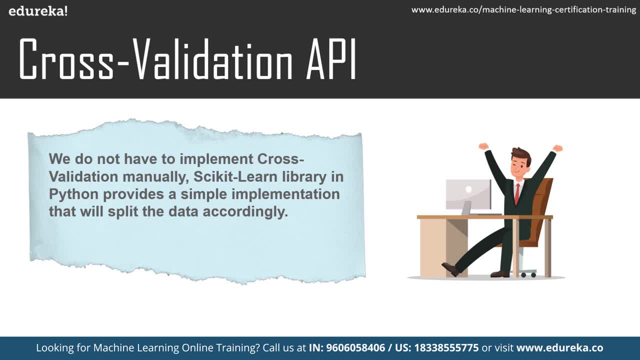 and then we have leave P out class stratified k-fold class as well. So just to show you, guys, let us try to use the k-fold, using python, to create training and validation sets. So for this I'll just do one thing, guys. first of all, 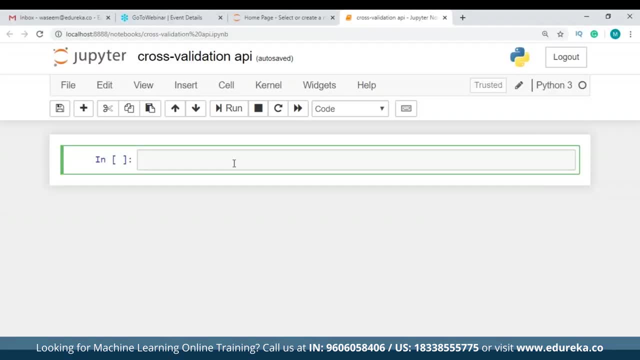 I'll just go to the Jupiter notebook over here. So we are in the Jupiter notebook guys. I'll do one thing. first of all. I'll import a few libraries, like I'll import the array from numpy and I will import Sk learn dot model selection. 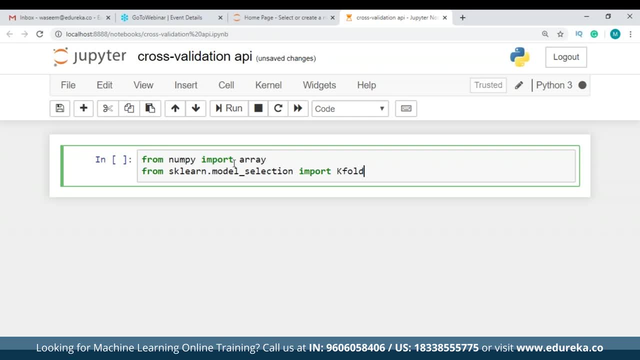 I am going to import K-fold. Okay, I made a mistake, I guess, so no errors here, guys. So first of all I have to sample my data, So I'll just take a area, So I'll take a row of a few numbers, since inside this, 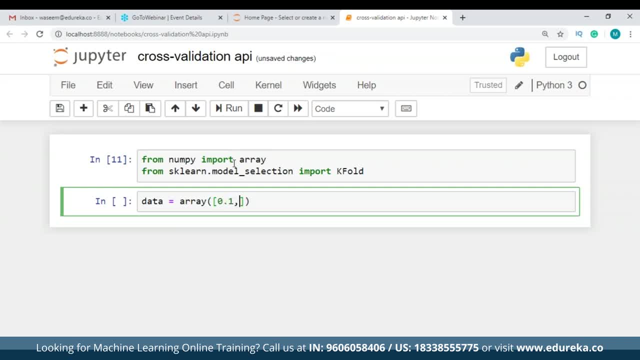 I'm just going to pass a list. So 0.1, let's say 0.2, 0.3, 0.4. So this is my data, guys. So now I have to split the data. for this I'm going to use the k-fold. 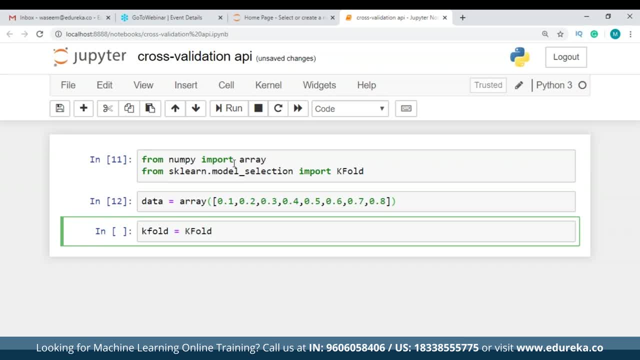 So I'll name it as k-fold only. I'll use the k-fold down and inside this I'll pass the data. So this is going to be with three. So I have to split my data into three. true, and I'll name it as one. 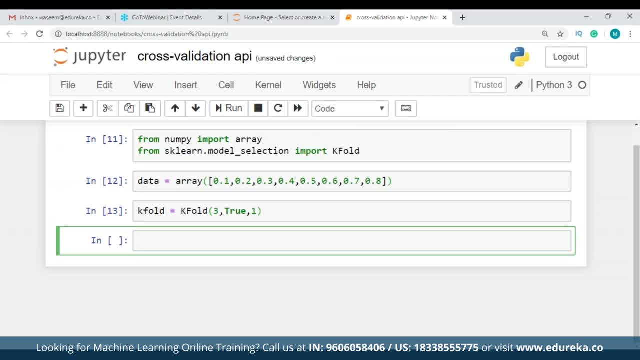 So no errors here as well. So now I'm going to enumerate my split. It's for that fun I'm going to take for loop and for train and test in, let's say, k-fold art splits. I'll pass data inside this and I'll just print. my train is equal to percentile s. 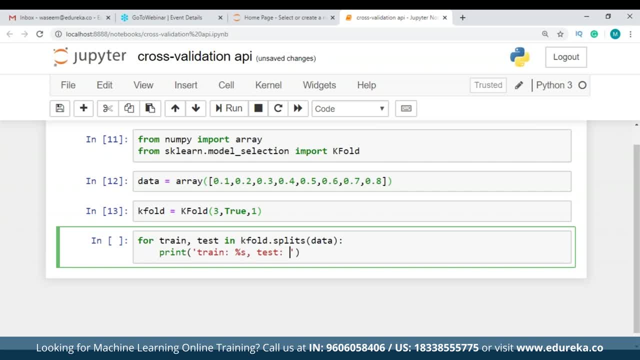 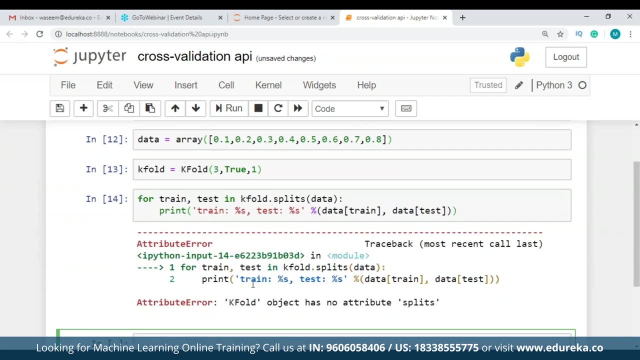 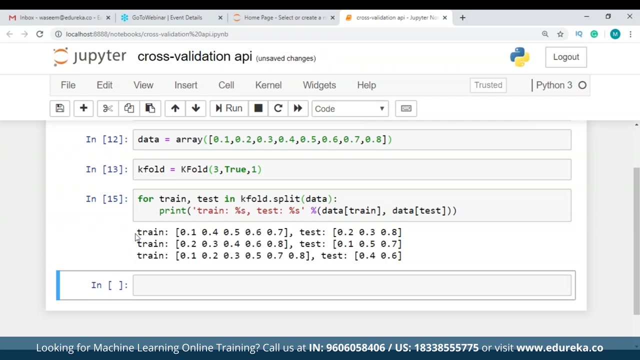 and test is equal to percentile s percentile Data, Train and data Test. so when I run this, okay, I have a attribute error. I write splits over here, So I'll just name it as split. So, as you can see, I have actually created a train. 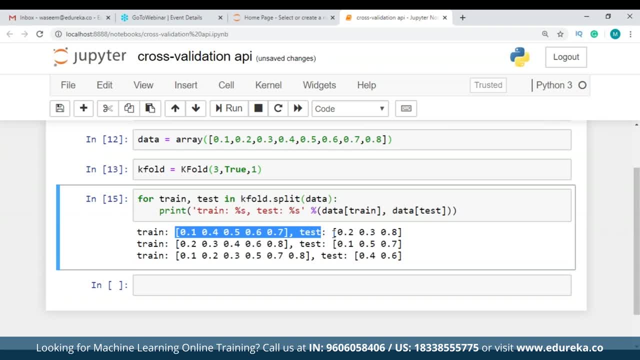 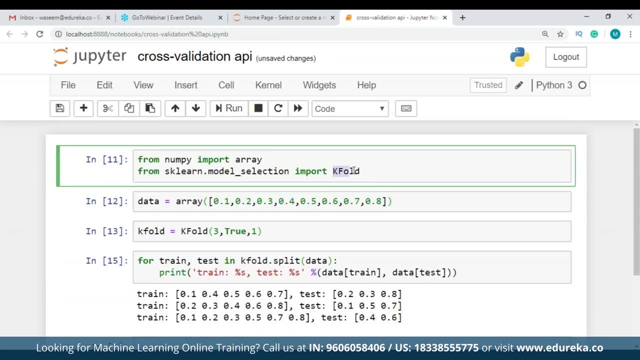 and test set using this data that I have over here. So this is how easily you can use a k-fold cross validation using the scikit-learn implementation, because we already have this k-fold class for implementing the k-fold cross validation and similarly we can choose other cross validation iterators. 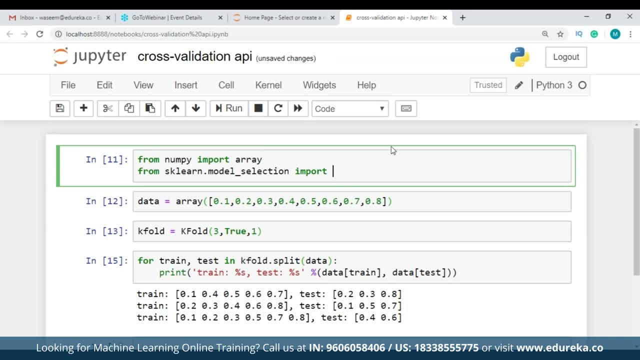 depending upon the requirement and the type of data. I'll show you what all we have. So we have leave one out, leave one group out, leave one out, leave P groups out. and we have leave P out, and then we have stratified, I guess. so we have stratified k-fold. 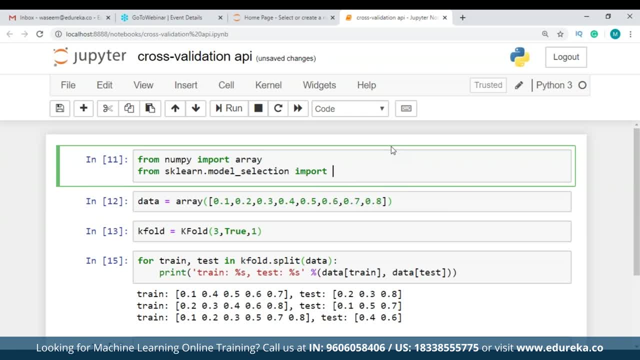 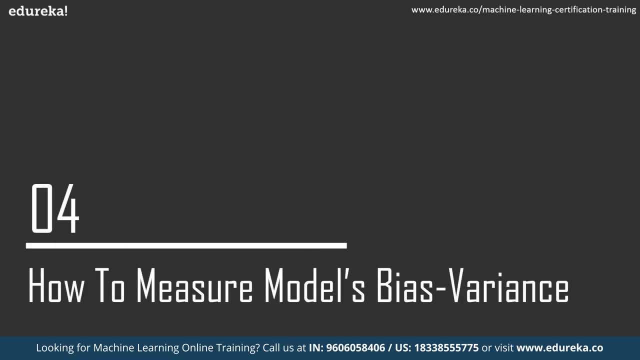 and stratified shuffle split as well. So there are a lot of different cross validation iterators that we can actually use. now, moving on, Let me tell you how we can actually measure the model's bias variance as well. So if we do the k-fold cross validation, 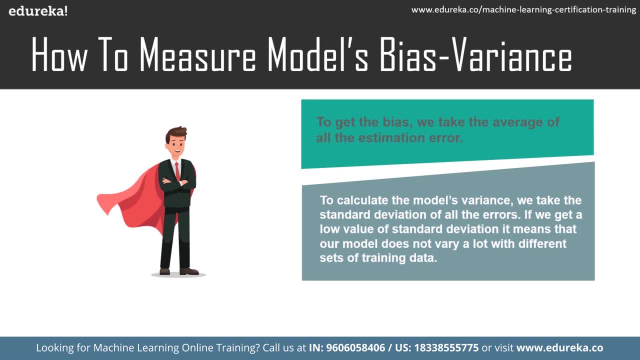 we will get K different estimation errors and in any ideal situation these error would sum up to 0. but it is quite highly unlikely to get such results and to get the bias. We just take the average of all the estimation error, So the model's accuracy is directly proportional. 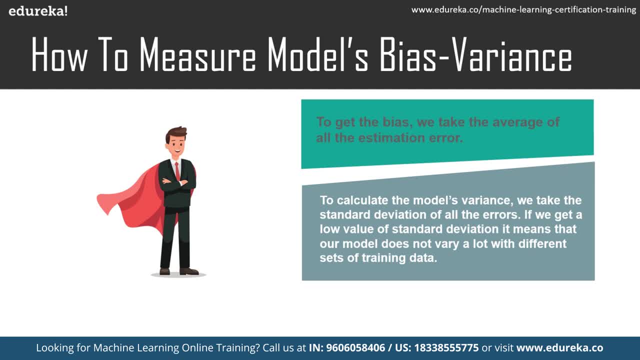 to the bias calculated. So the model's accuracy is quite proportional to the bias calculated. and to calculate the model's variance We take the standard deviation of all the errors. So if we get a low value of standard deviation it means that our model does not vary a lot. 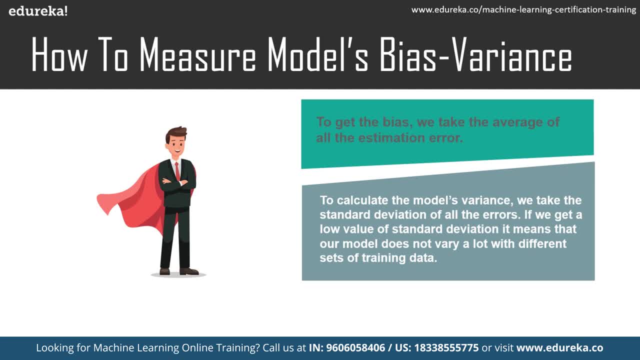 with the different sets of training data, and the focus should be to maintain a balance between the bias and the variance of the model. This can be achieved by reducing the variance to the minimum and controlling the bias, and this trade-off usually results in making a better predictive model. 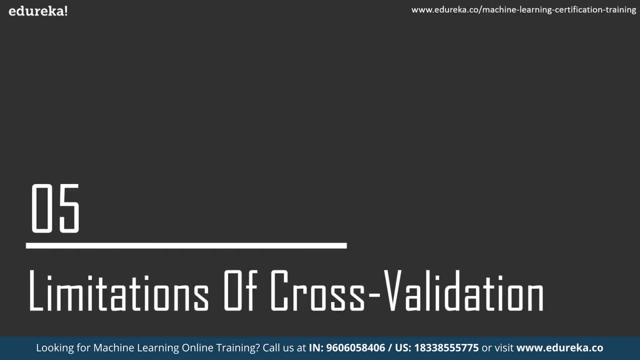 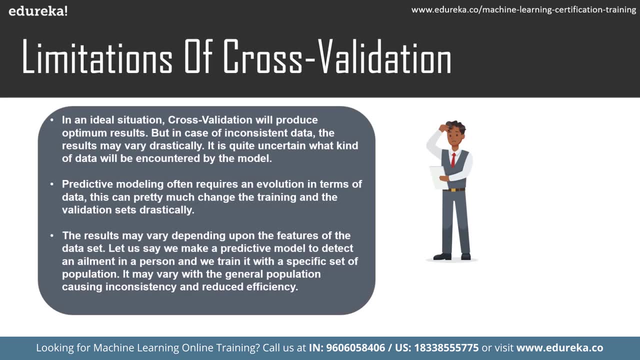 but there are a few limitations with cross validation as well. So let's take a look at various limitations with cross validation as well. So these are a few limitations that are faced by cross validation. So in an ideal situation, cross validation will produce optimum results. 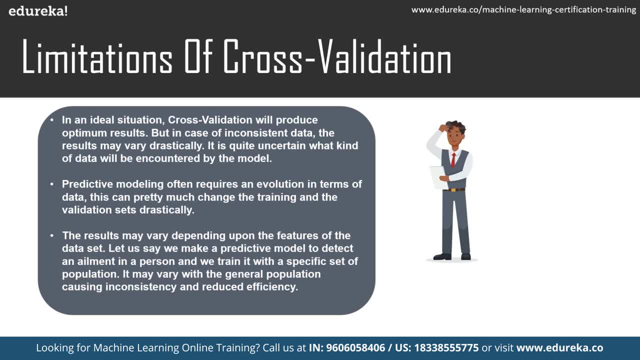 but in case of inconsistent data, the results may vary drastically. It is quite uncertain What kind of data will be encountered by the model. So that is one limitation we have with cross validation. The next one is predictive modeling often requires an evolution in terms of data.